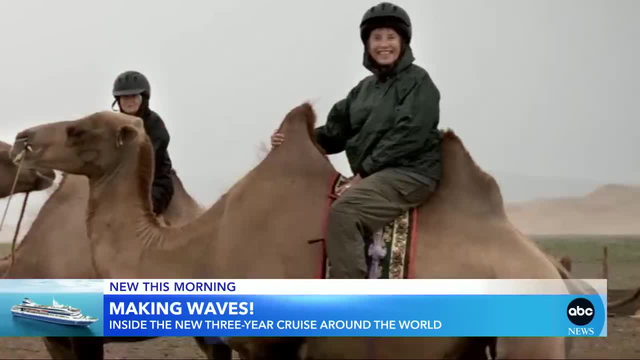 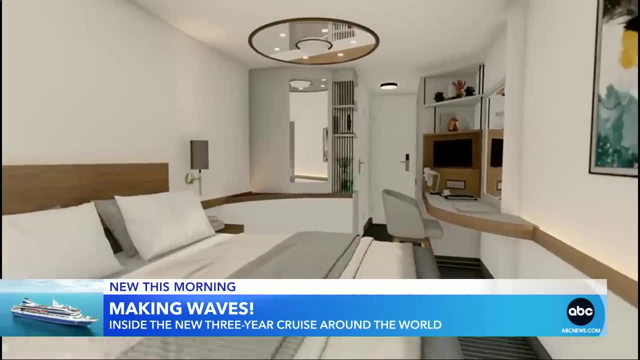 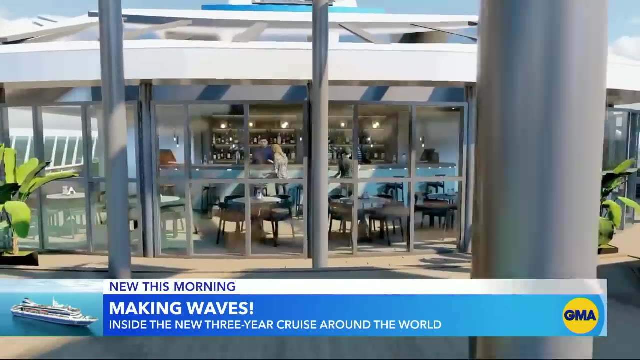 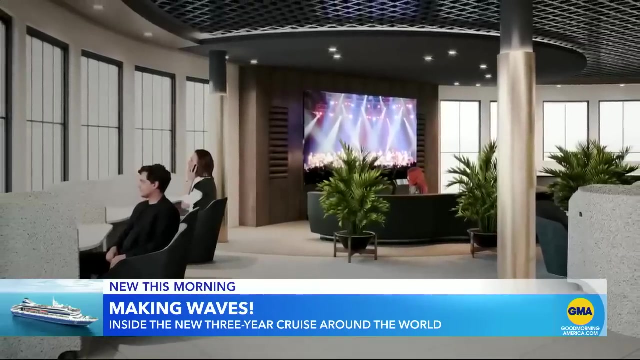 flight attendant booked one of the biggest rooms on the ship. She's hoping for the experience of a lifetime. This is going to be the perfect place to do it all. Here's what a typical state room will look like Right now. it costs $33,000 per year, which includes food, some drinks, entertainment and a fitness center. And this three-year tour is not just for retirees. The ship is wired for professionals working remotely, with meeting rooms, offices, a library and Wi-Fi. 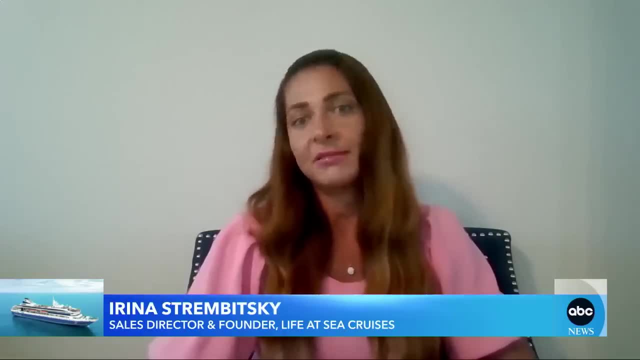 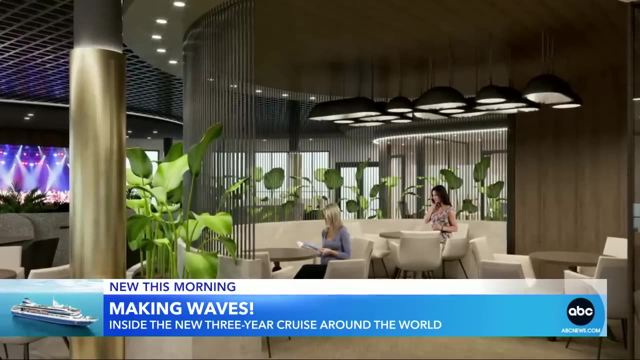 We're looking at half the ship. The ship is under 60. And that was a huge surprise to me. And now the people are getting younger and younger with each day. We're getting more and more people in their 20s with each day. 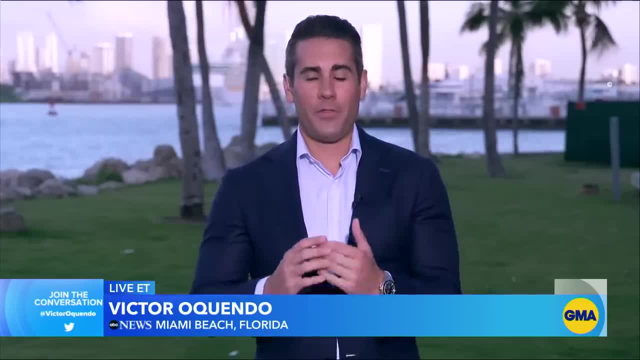 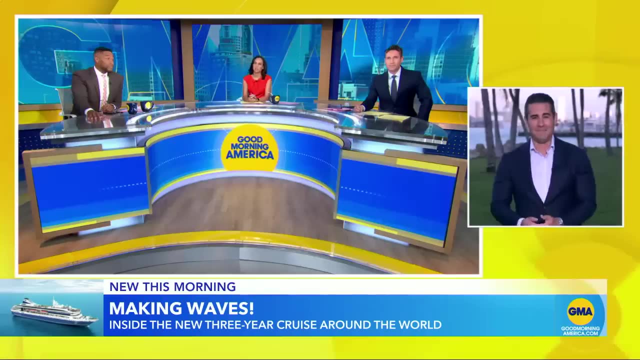 And there is no one or two-year option here. This is for a full three years, But if you're ever feeling homesick, you can have friends or family stay in some of the guest cabins for free. Guys, That's just what we need. Thanksgiving, come on over. 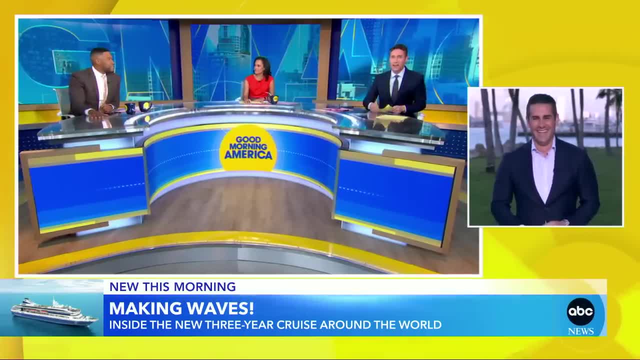 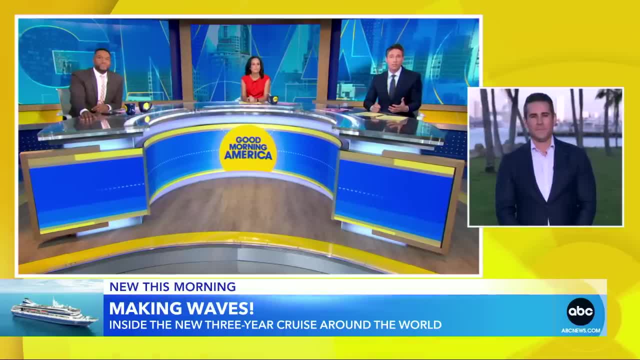 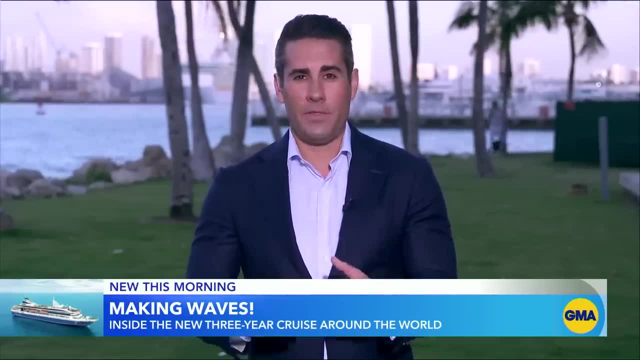 It looks like they are coming back much stronger now. Can people still find deals out there? They absolutely can, And it all depends on when you book. There are deals on cruises in the first few months of the years, But those fares start to climb as we approach the busy summer travel season. 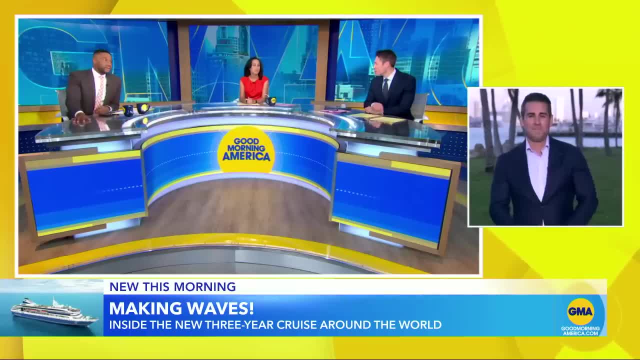 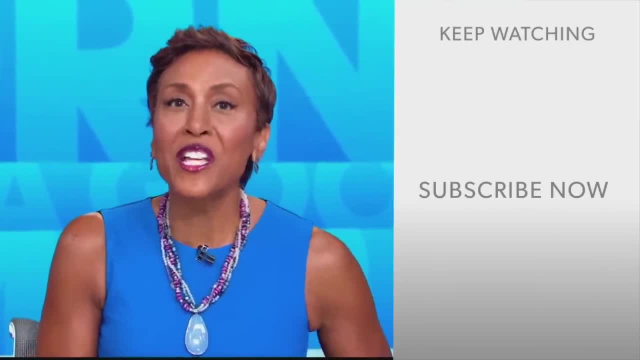 So now is the time to book Guys. Start with three days And then maybe we'll get to three years after that. Well, hey there, GMA fans, Robin Roberts here. Thanks for checking out our YouTube channel. Lots of great stuff here. 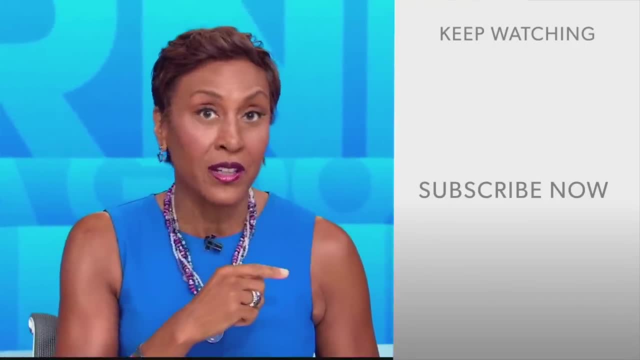 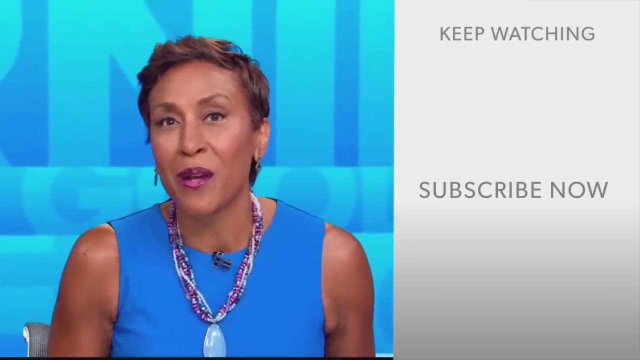 So go on, click the subscribe button right over here to get more of awesome videos and content from GMA every day, anytime. We thank you for watching and we'll see you in the morning on GMA.